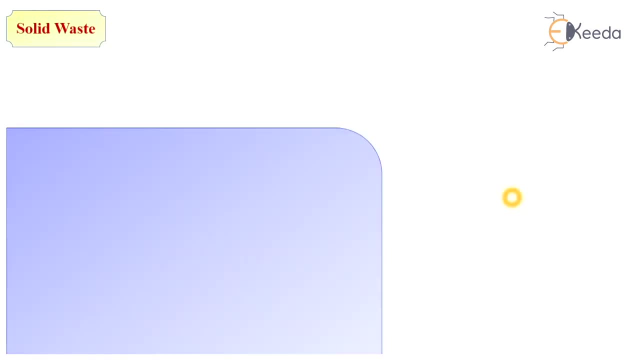 So these are different types of waste. So now we are focusing on solid waste. So what is solid waste? So solid waste is defined as it is non-liquid, non-soluble material, ranging from municipal garbage to industrial waste. 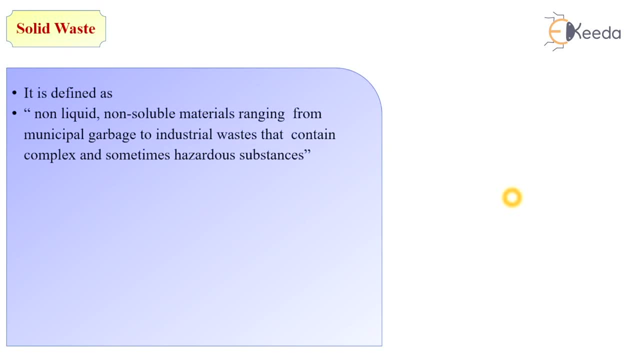 that contain complex and sometimes hazardous substances. So, most important, the solid waste is non-liquid and non-soluble waste. So solid waste also include garbage, rubbish, demolition product, sewage treatment residues, dead animals or manure and other discarded materials. 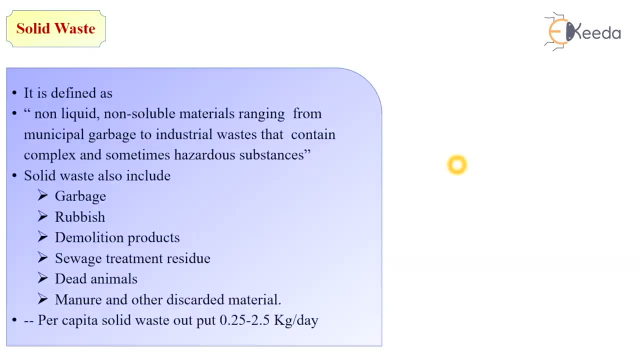 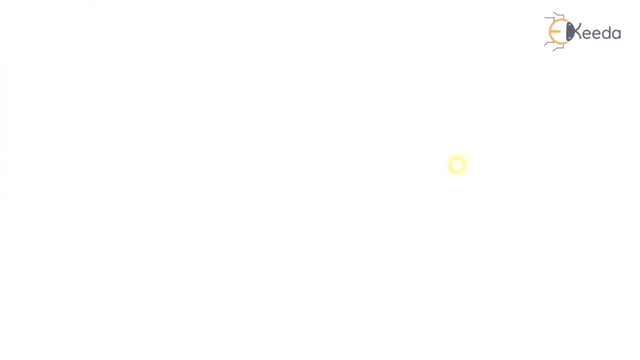 So generally the per capita solid waste generation rate is 0.25 to 2.5 kg per day. So different sources of solid waste are. the solid waste is generated either from agricultural activities or fisheries, or household activities, or commercial or industrial activities. 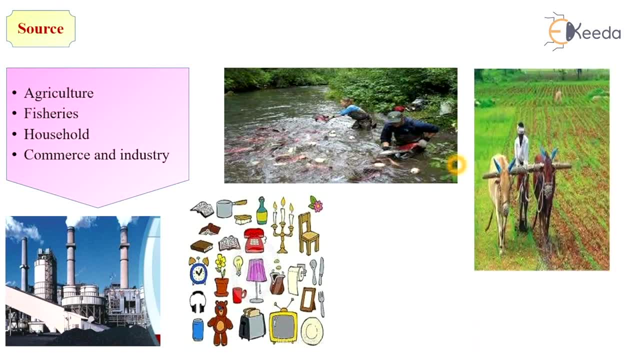 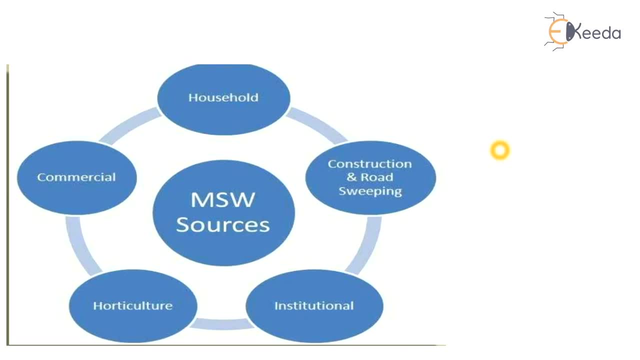 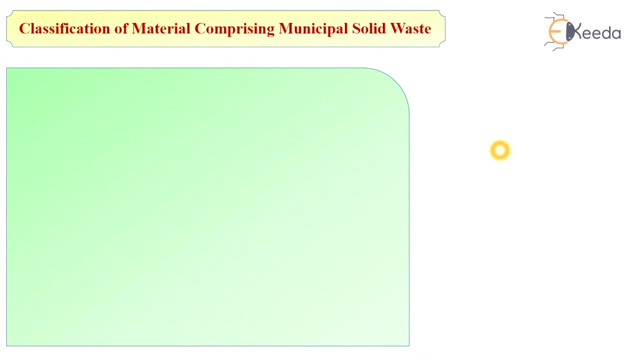 So, as you can see in these images, So the municipal solid waste sources are from household construction waste, institutional waste, agricultural or horticultural waste and commercial waste. So the classification of solid waste, of material comprising municipal solid waste, 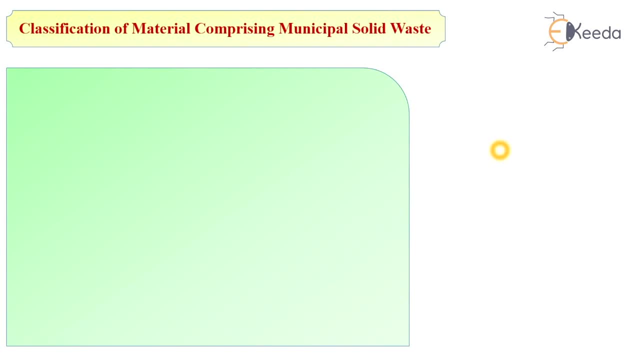 Again, municipal solid waste is a part of solid waste that we have already seen. The solid waste is a part of solid waste that we have already seen. So the solid waste is divided into types of waste, that is, municipal solid waste, commercial solid waste, industrial solid waste, hospital waste, etc. 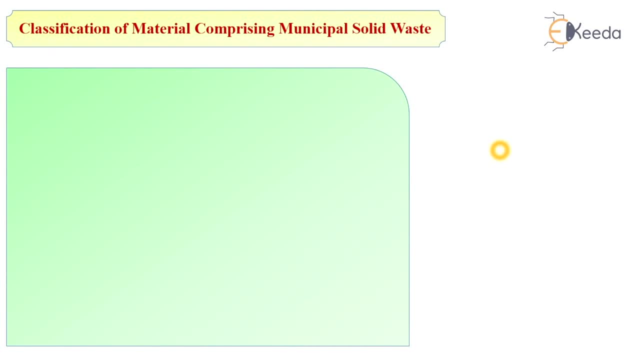 So municipal solid waste is a part of solid waste. So now we are going to see the classification of material or content which are present in municipal solid waste. So municipal solid waste consists of: first is garbage. So what is garbage? 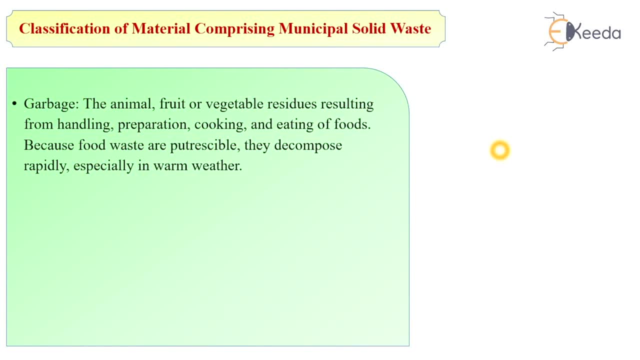 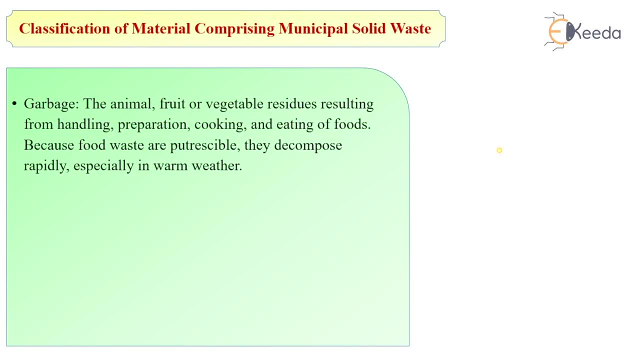 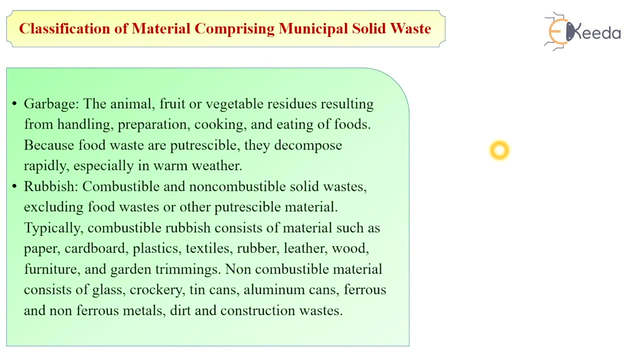 they decompose rapidly, especially in warm weather. So next content present in municipal solid waste is rubbish. So what is rubbish? The combustible and non-combustible solid waste, excluding the food waste, because food waste comes under category of garbage. 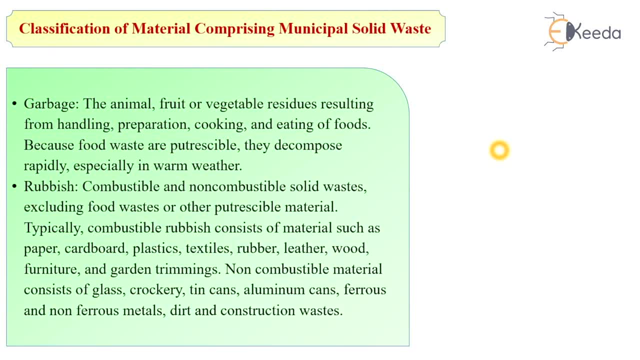 So excluding the food waste or other putrescible material. Typically combustible rubbish consists of materials such as paper, cardboard, plastic, textile, rubber, leather, wood, furniture pieces and garden trimmings, And non-combustible material consists of glass, crockery, tin cans, aluminium cans, ferrous and non-ferrous metals, dirt and construction waste. 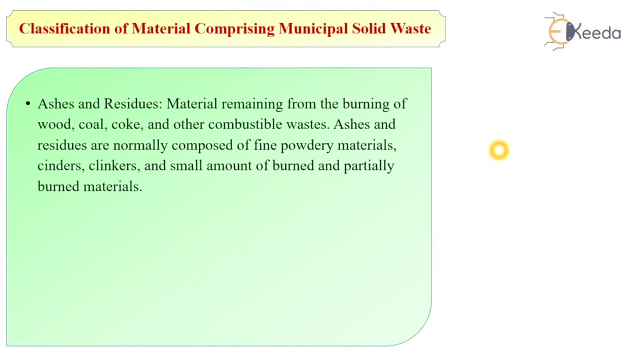 So again, the next content present in municipal solid waste are ashes and residues, The material remaining from burning of wood, coal, oak and other combustible waste, which are classified under ashes and residues. The ashes and residues are normally composed of fine powdery material, cinders, clinkers and small amount of burnt and partially burnt materials. 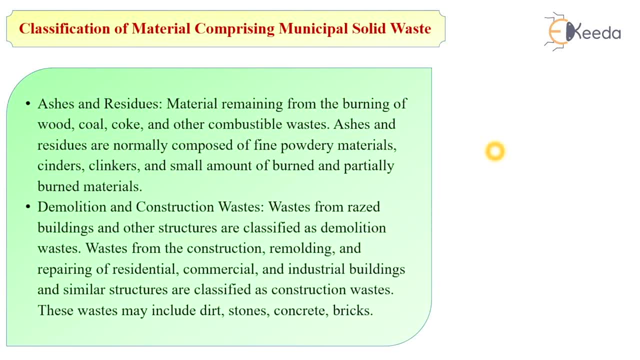 Next is demolition and construction waste. The waste from raised buildings and other structures are classified under demolition waste. Waste from the construction, remoulding, repairing of residentials, commercial buildings, commercial and industrial buildings and similar structures are classified as construction waste. 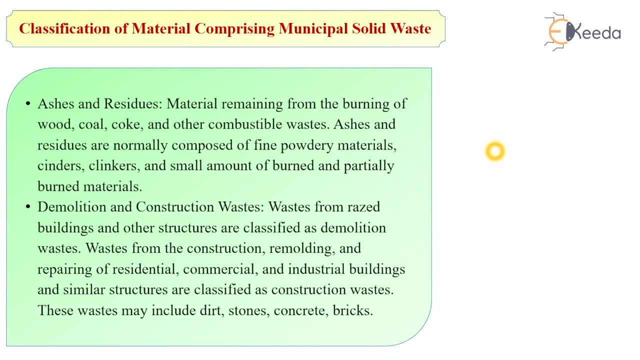 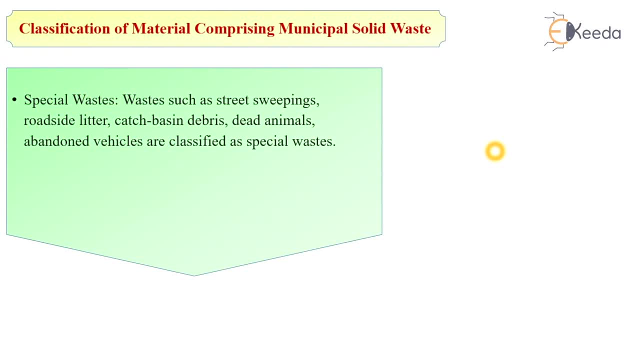 These wastes may include dirt, stone, concrete bricks, etc. Next is spatial waste. The wastes such as street sweepings, roadside litters, catch basin debris, dead animals, abandoned vehicles are classified under spatial waste. And last is trickery. 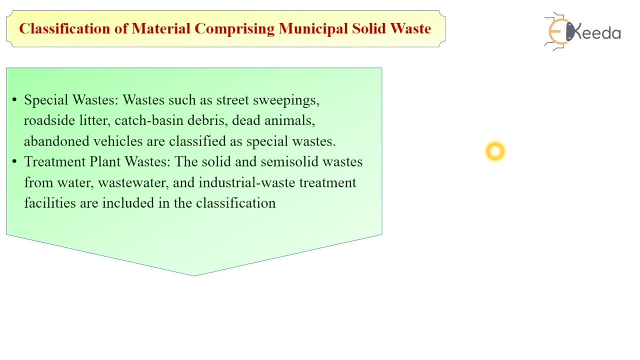 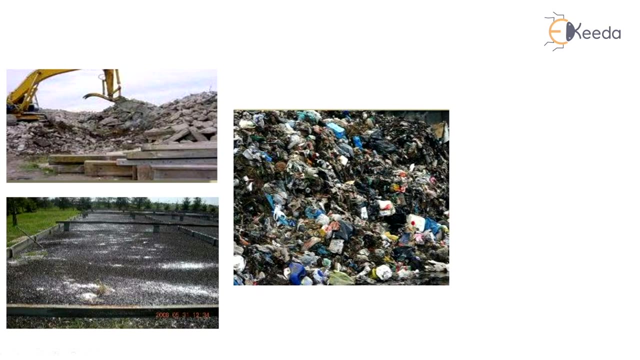 Precip. Straight tacks and tacks are classified as treatment waste. The solid and semi-solid wastes from water waste and industrial waste treatment facilities are included in the classification of treatment waste. So as you can see in this figure. So this first image represents the demolition waste. 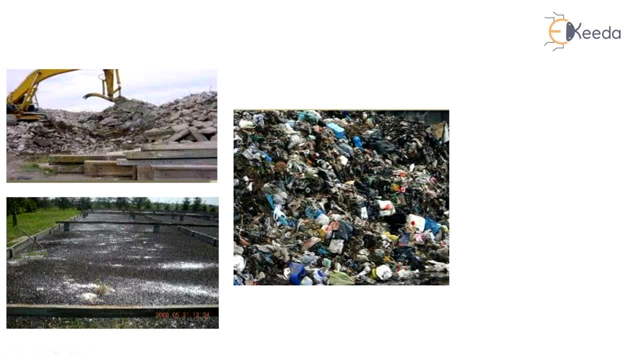 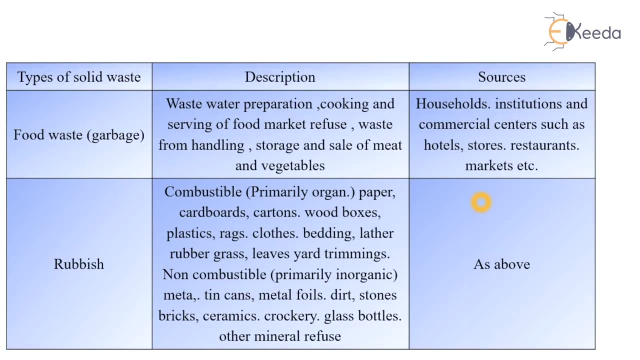 The second one is garbage And this one is some roadside waste. So these are different kind of material and contents that are present In municipal solid waste. So, as you can see in this figure, solid waste or that are the parts of municipal solid waste. So this is the tabular form. 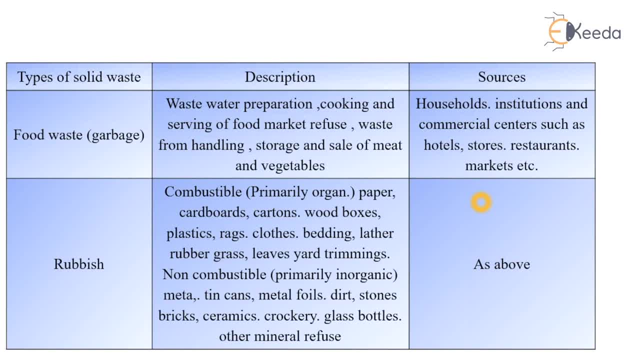 of contents or types of municipal solid waste that we are already seen. we have already seen. So if the question ask in your examination, either you can write this question answer in theoretical or paragraphical form or in tabular form. So this contents or the theory. 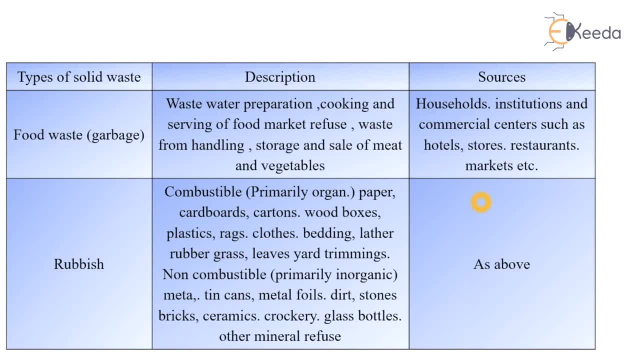 is similar to previous one. So let's we see the types of municipal solid waste. First, we have already seen the garbage. Garbage is wastewater preparation, cooking and serving of food, market refuse, Waste from handling, storage and sale of meat and vegetables. The 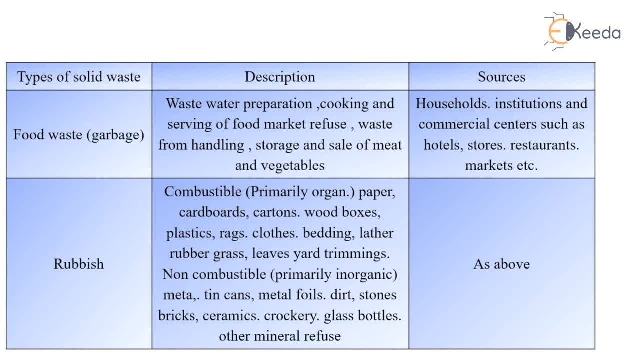 sources of garbage or food waste are generated from household and institutional and commercial activities, such as hotels, stores, restaurants, markets, etc. Next is rubbish. The rubbish are the combustible materials, such as paper, cardboard cartons, wood boxes, plastics, rags, cloths, beddings, leather, rubber, glass, leaves, yard trimmings. 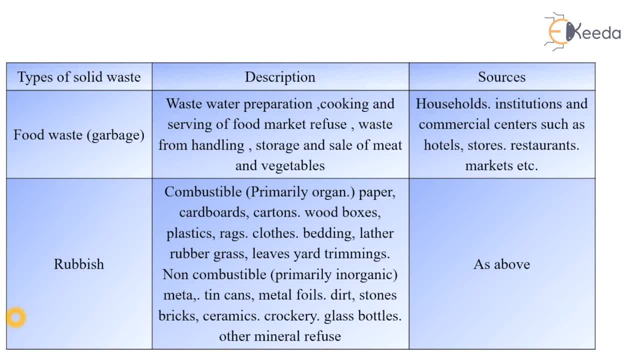 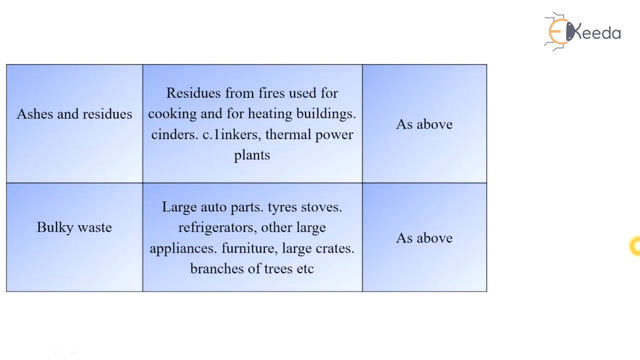 etc. and non-combustible materials such as metal, tin cans, metal foil, dirt, stone bricks, ceramics, crockery, glass bottle and other mineral refuges. So source of the rubbish is either from some construction material or from commercial activities. 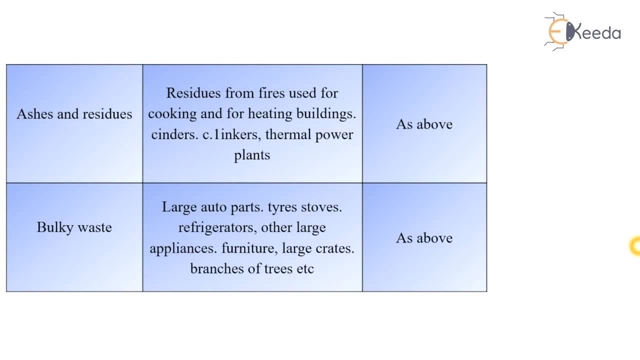 Next is ashes and residues: The residues from fires used for cooking and for heating buildings, cinders, clinkers, thermal power plant, etc. And the bulky waste is consist of large auto parts, tires, stoves, refrigerators parts and other things. So this is the waste that 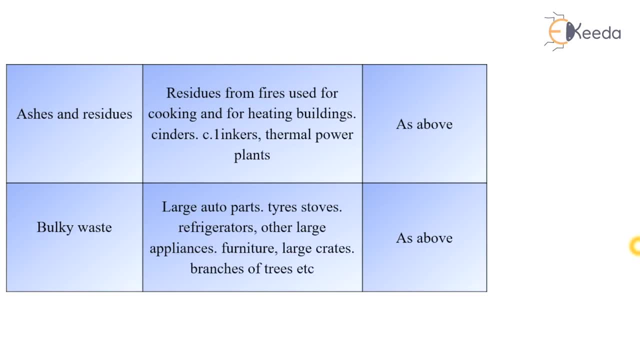 is used for cooking and for heating buildings. So this is the waste that is used for cooking and for heating buildings. So this is the waste that is used for cooking and for heating centers and other large appliances, furniture, last crates, branches of trees, etc. are comes. 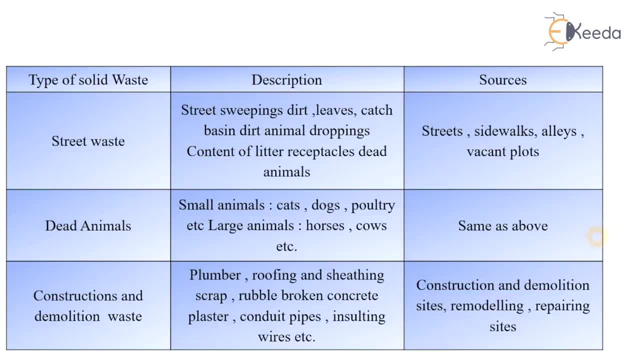 under bulky waste. Next is street waste. Street sweeping, dirt, leaves, catch, basin debris, animal droppings, content of litter receptacles, dead animals etc. And sources of street waste are from street sidewalks, alley, vacant plots etc. 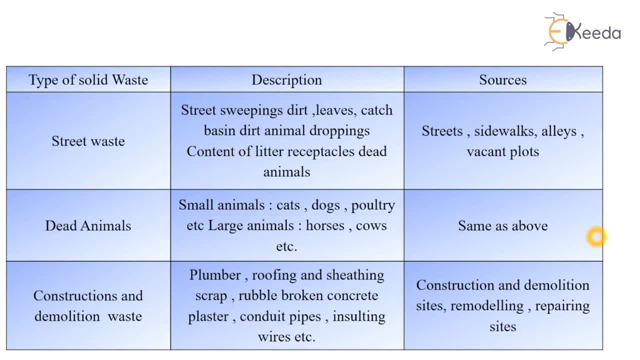 Next is waste whose size is almost like the frame that close under them, A waste used for flower nursery veure così travelled. there are few others. light wont to be wasted is dead animal waste: the small animal- cat, dogs, poultry, etc. and large animals- horses. 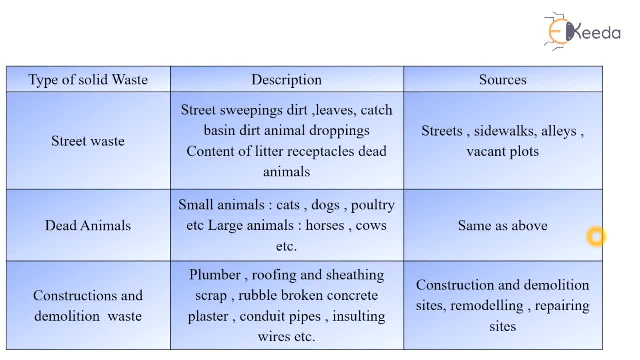 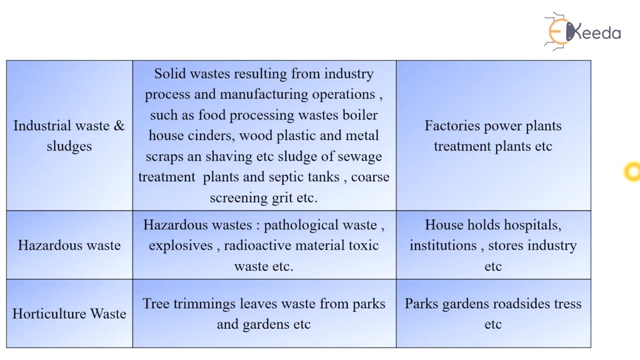 cows, etc. And last one is construction and demolition waste, which is classified under plumber, roofing material, sheeting scraps, rubble, broken concrete, plasters, conduit pipes, insulating material, wires, etc. and source are from construction and demolition sites remoulding repairing sites. Next is industrial and sludge waste of different 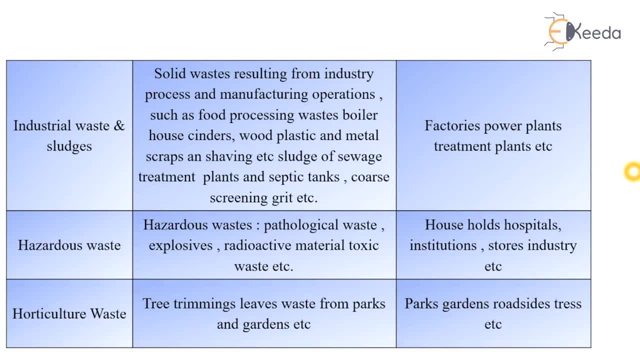 water and wastewater treatment plants, The solid waste resulting from industry process and manufacturing operations, such as food processing waste, boiler house cinders, etc. wood, plastic and metal scraps and shaving, etc. sludge of sewage treatment plant and septic tank hose screening grid, etc. And the sources of this industry are from: 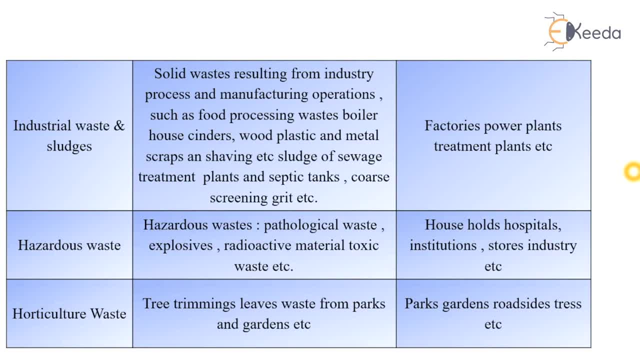 industrial waste and sludges are from different factories, power plants, treatment plants, etc. Next one is hazardous waste. Hazardous waste consists of pathological waste, explosives, radioactive waste, toxic waste, etc. And sources of generation of hazardous waste are from some household activities: hospitals, institutions, stores, industries, etc. Next is horticultural. 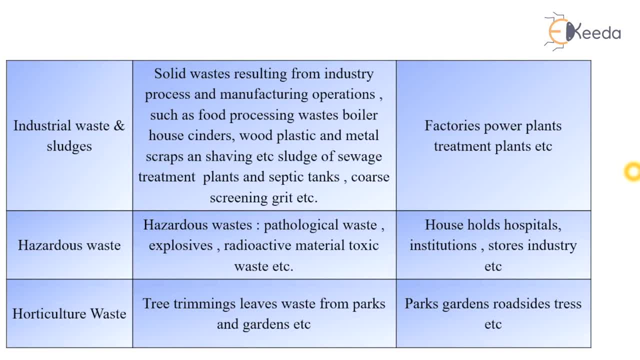 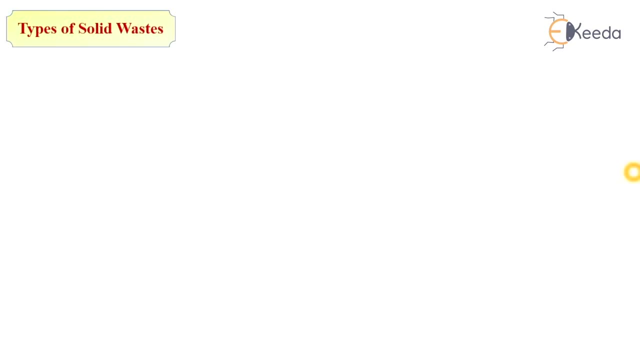 waste The tree trimming leaves, waste from parks and gardens are comes under horticulture waste And sources are from parks, gardens, roadside trees, etc. So now we have seen the types or classification of particular municipal solid waste. So now we are seeing the classification or types of in general solid waste. 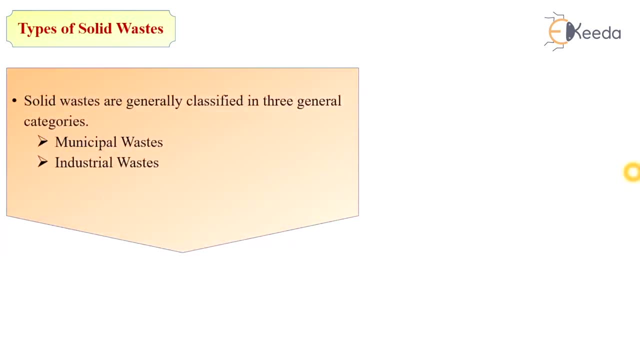 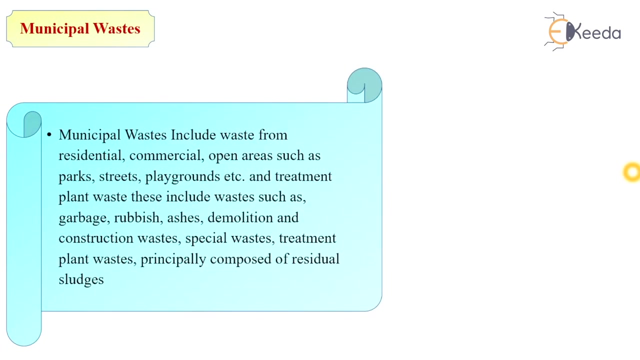 So we have already seen the classification of municipal solid waste. So what is municipal solid waste? Municipal waste include waste from residential, commercial, open areas such as parks, streets, playgrounds, etc. And treatment plant waste. this includes waste such as garbage. 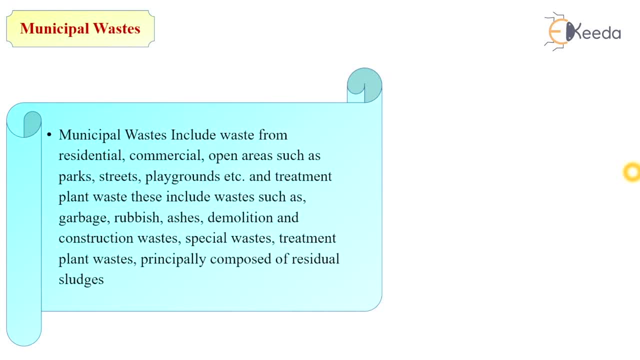 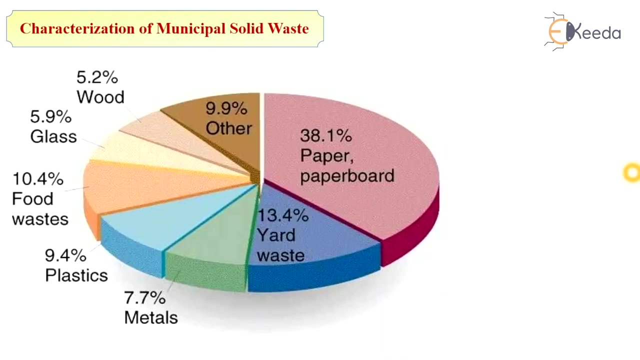 rubbish, ashes, demolition and construction waste, special waste, treatment plant waste principally composed of residual sludge, etc. So we have already seen the classification of municipal solid waste. The garbage, rubbish, demolition waste, industrial wastewater comes under this municipal solid waste. So next type of solid waste is industrial waste. So 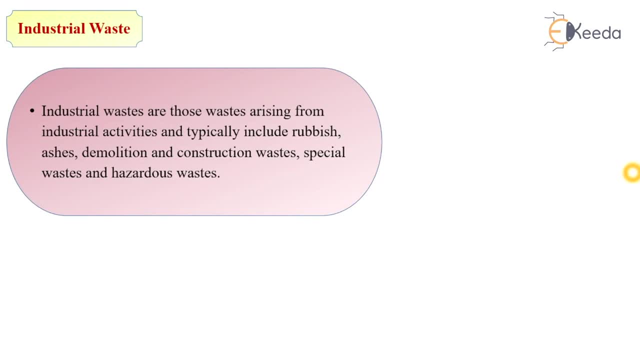 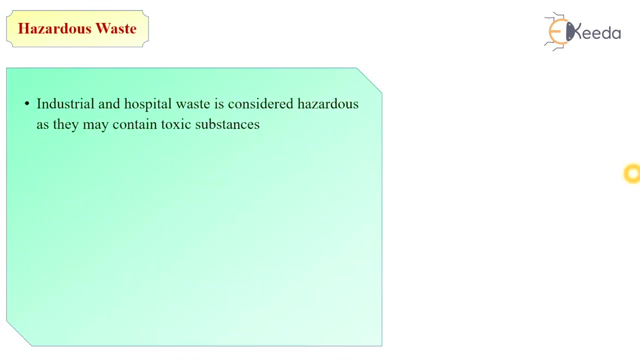 industrial waste includes waste from agricultural work-use and equipment collection, such as garbage, are those wastes arising from industrial activities and typically include rubbish, ashes, demolition and construction waste, special waste and hazardous waste. So next type is hazardous waste. The industrial and hospital waste is considered under hazardous. 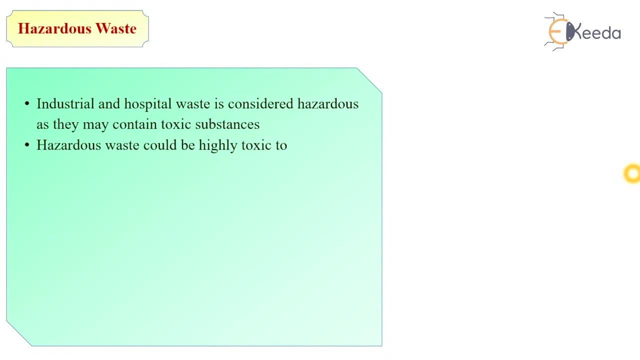 as they may contain different toxic substances, The hazardous waste could be highly toxic to humans, animals and plants. They are corrosive, highly inflammable or explosive. In the industrial sector, the major generators of hazardous waste are the metal, chemicals, papers, pesticides, dye, rubber and different industrial products. 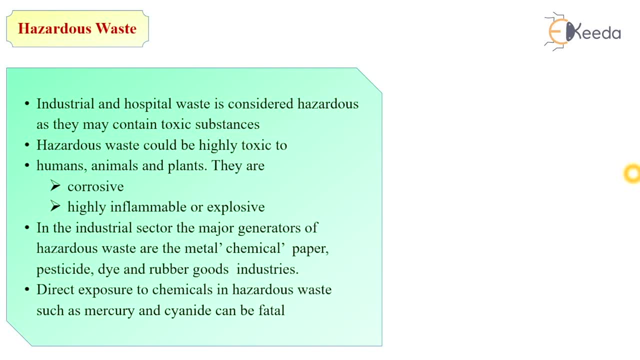 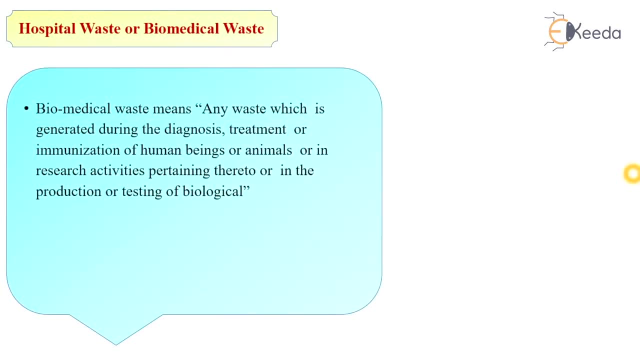 So direct exposure to chemicals in hazardous waste, such as mercury and cyanides, can be factor. So next is hospital waste, So next is hospital waste. So next is hospital waste, or biomedical waste, which is also comes under hazardous waste. The biomedical waste means any waste which is generated during the diagnosis treatment. 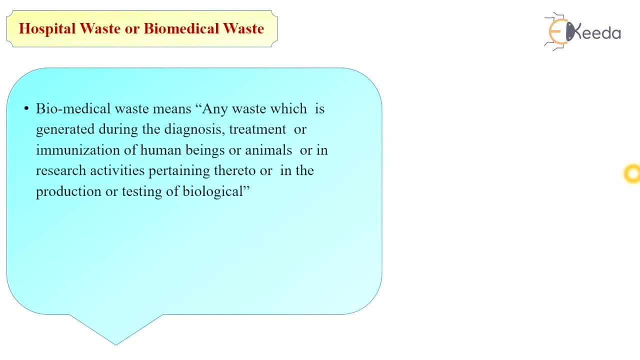 or immunization of human being or animals, or in research activities pertaining thereto, or in the production or testing of biological activities. So it may include waste like sharp waste, pathological waste, pharmaceutical waste, geotextile, genotextile waste, chemical waste and radioactive waste. 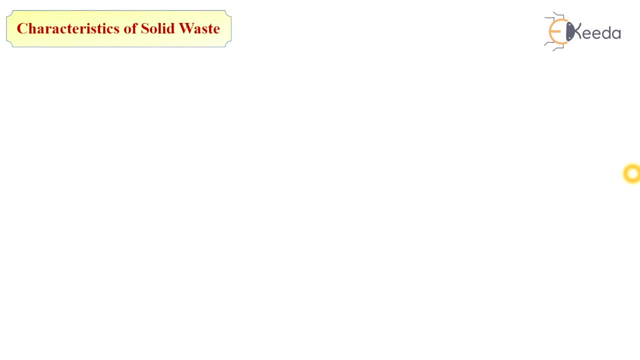 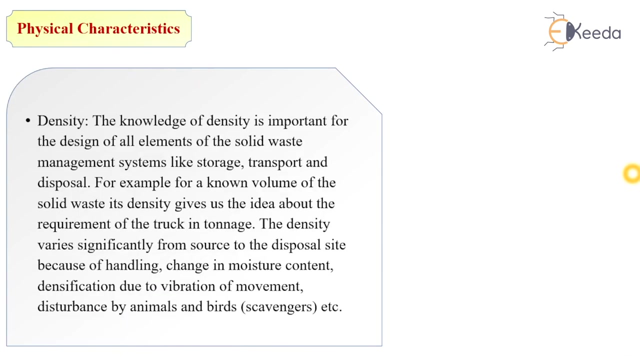 So next important is characteristics of solid waste. So, similar to characteristics of water and waste water, the solid waste have some different characteristics. So again there are physical and chemical characteristics. So under physical characteristics, the first one is density. The knowledge of density is important for the design of all element of the solid waste management system, like storage, transport and disposal of solid waste. 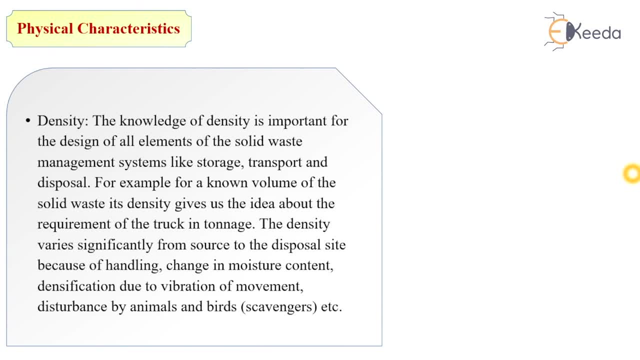 For example, for a known volume of solid waste, its density gives us the idea about the requirement of the truck. in tonnage, The density varies significantly from soil to water. The density varies significantly from source to disposal site because of handling change in moisture content. 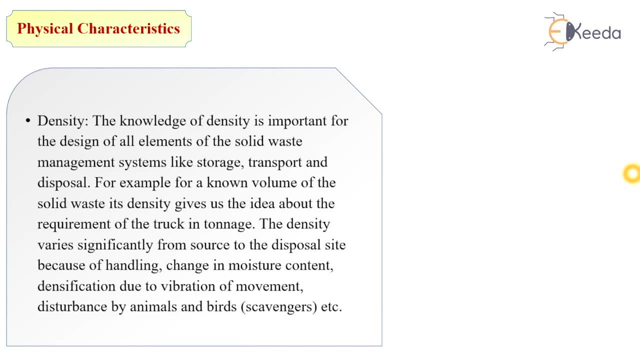 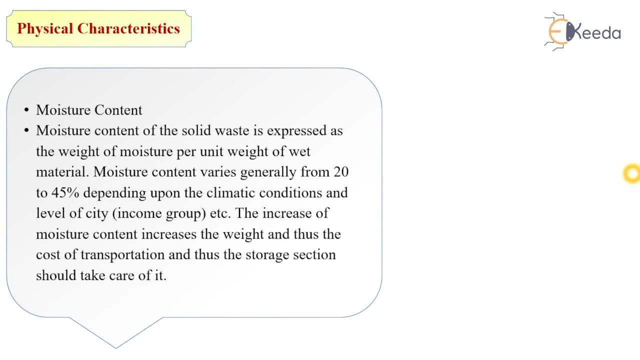 densification due to vibrations of movement, disturbances by animals and birds, etc. So the density of solid waste varies from part to part. The next physical characteristics is moisture content. Moisture content of the solid waste is expressed as the weight of the solid waste. 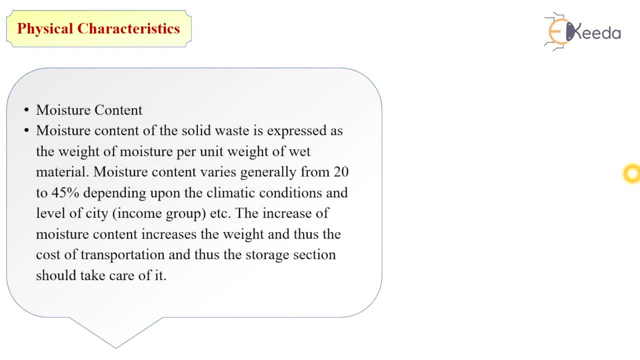 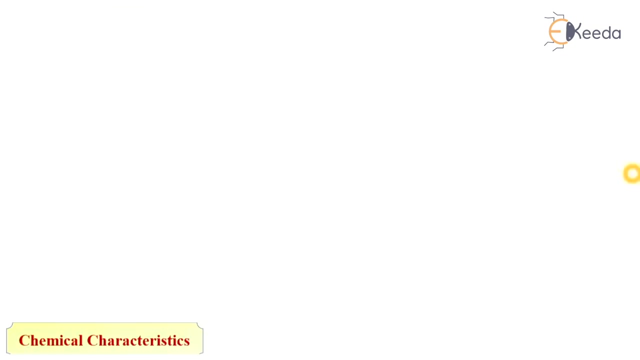 The moisture content varies generally from 20 to 45%, depending upon the climatic conditions and level of city, etc. The increase of moisture content increases the weight and thus cost of transportation, and the storage section should take care of it. So next are chemical characteristics. 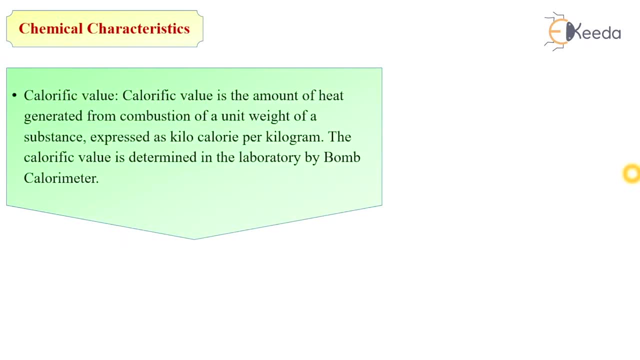 So first is calorific value. What is calorific value? The calorific value is the amount of heat generated from combustion of a unit weight of substances, expressed as kilocalories per kilogram. The calorific value is determined in the laboratory by Bohm calorimeter. 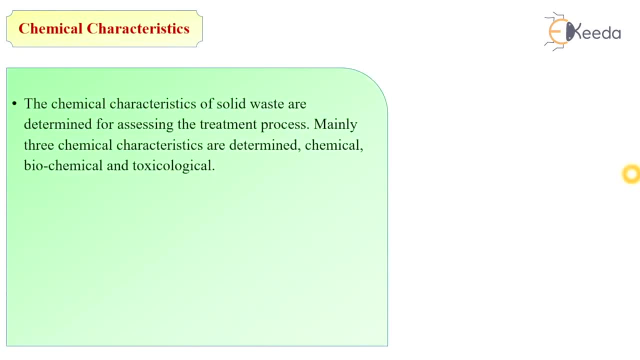 Next, chemical characteristics of solid waste are determined of assessing the treatment process. Next, chemical characteristics of solid waste are determined of assessing the treatment process. Mainly three chemical characteristics are determined: Chemical, biochemical and toxicological. The chemical quantities of solid waste in Indian urban centers are pH, nitrogen, phosphorus, potassium. 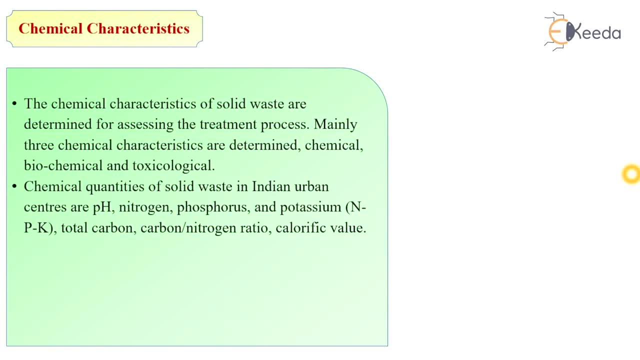 So that is NPK count, the total carbon carbon nitrogen ratio and calorific value. So these are comes under chemical characteristics. So these are comes under chemical characteristics. Biochemical characteristics include carbohydrates, proteins, as well as biodegradable environmental elements. 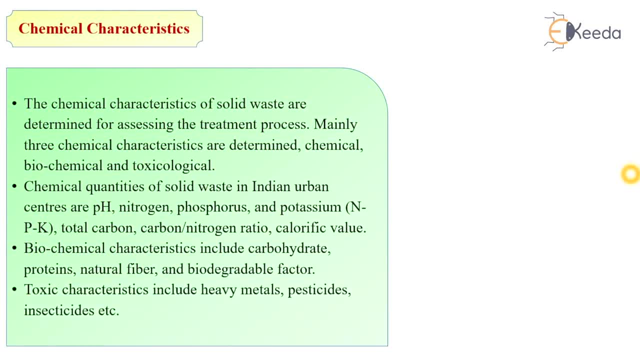 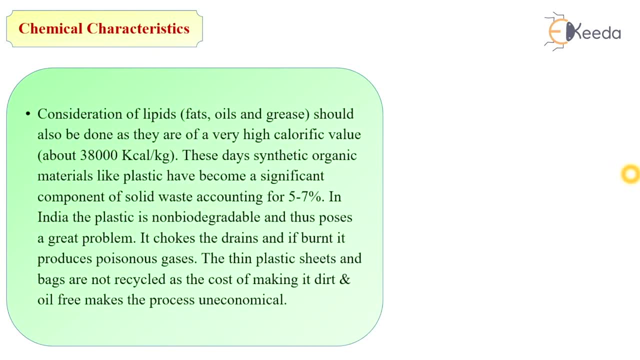 Also toxic characteristics- includes heavy metals, pesticides, insecticides, etc. Again, the consideration of lipids, ie fats, oil and grease are also important- should also be done as they are of very high calorific value, ie about 38,000 kcal per kg of solid. 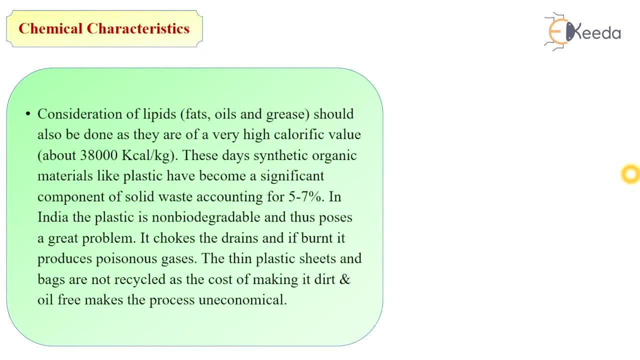 These days, the synthetic organic material like plastic have become a significant component of solid waste, accounting for 5-7% In India. the plastic is non-biodegradable and thus possesses a great problem: It chokes the drains and it burns. it produces poisonous gases. 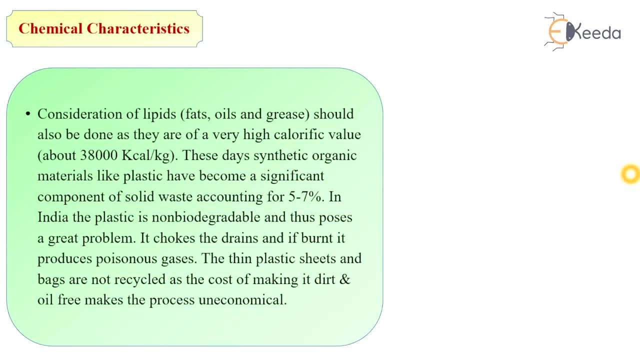 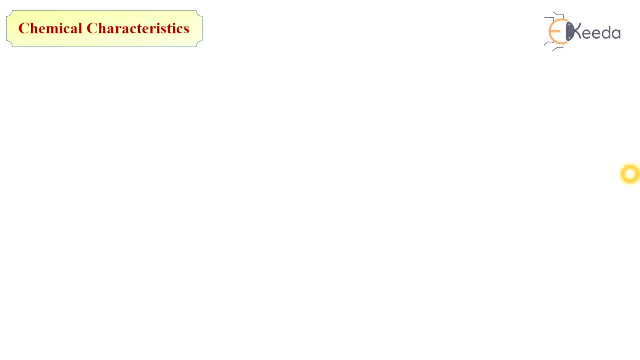 The thin plastic sheets and bags are not recycled as the cost of making it dirt and oil free make process uneconomical. So all the above considerations of characteristics are required to design, conceive and assess the most appropriate way of transportation. The requirements of treatment.